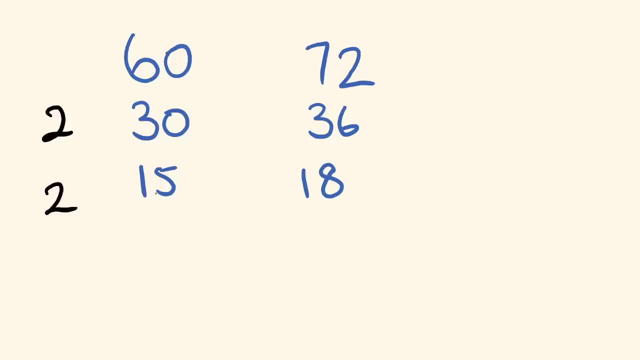 Okay, Is there any number that goes into both of these? All right, three does, Three goes into this one five times and it goes into this one six times. Now, is there any number that goes into both of these? Oh, you could say, yeah, one does, but one won't reduce the number anymore. 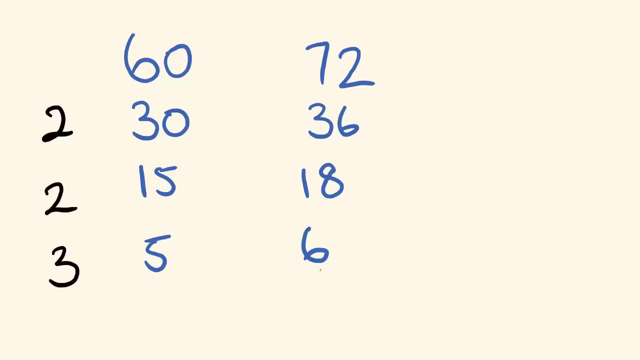 So we've hit this stage where these we have a couple of our numbers here where they can't be reduced anymore. So we look at these three numbers- the two, the two and the three- and we multiply these together to get the number. 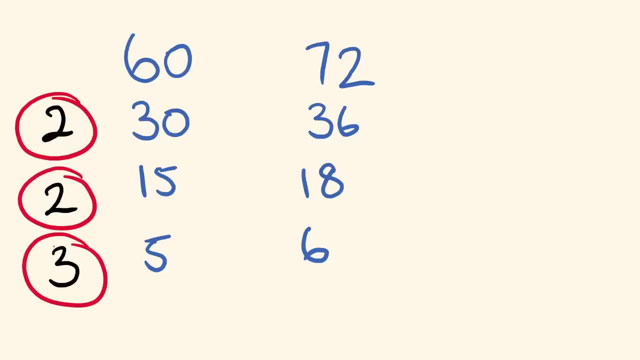 We multiply these together to get that greatest common factor. Two times two is four times three. our greatest common factor is 12.. Pretty easy, right? Okay, let's have a look at another one of these. Okay, so say, we want to work out the greatest common factor. 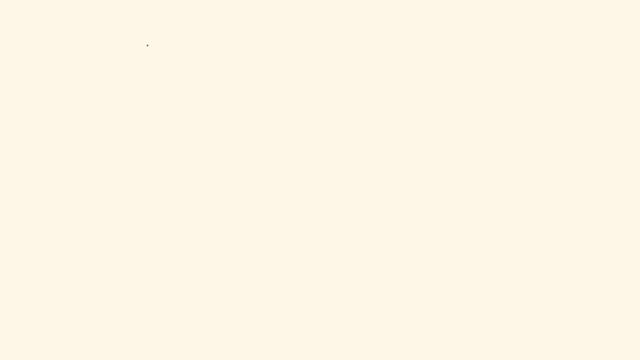 Let's have a look at what about 72 and 108.. Okay, you might even give this a go So you could look at these straight away and you could possibly recognize that nine goes into both of these. Okay, so you could be like, okay, nine goes into this one. 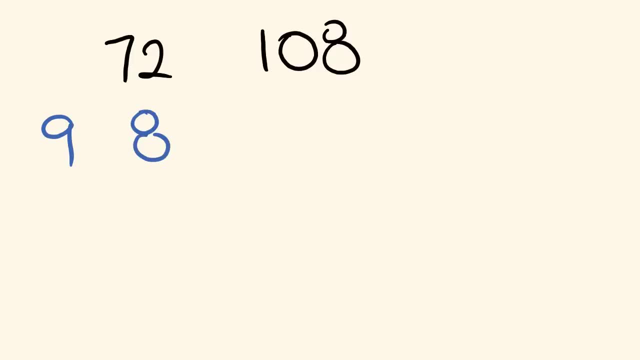 Okay, nine eight is 72, and 12 times nine is 108.. Okay, so that's our first number. We've got the next ones. Is there any number that goes into both of these? Yeah, okay, four does. 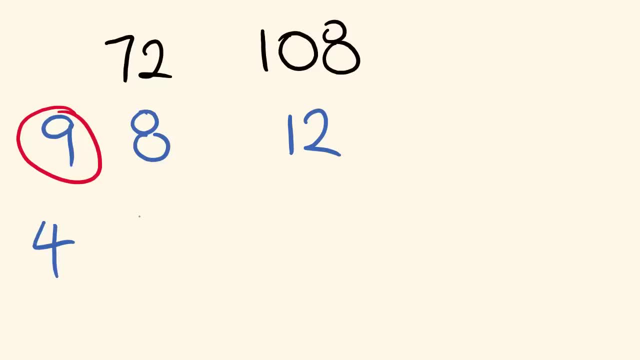 Four goes into this one two times and it goes into this one three times. Okay, And is there any numbers that go into both of these? Hey, there's not. So we multiply these two numbers through nine times four. Our highest common factor is 36.. 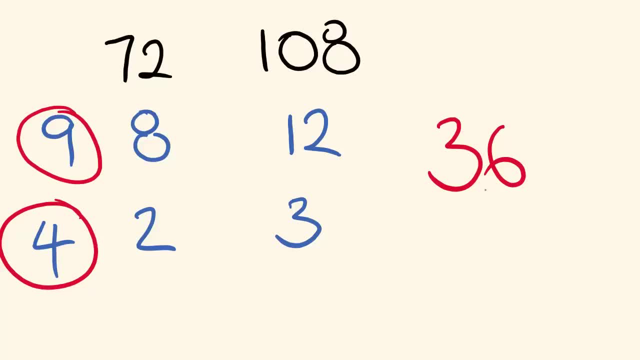 Anyway, I don't know what you think of that video. I hope you liked it. It's a fairly quick and easy way of doing this Without getting into messy factor trees. I always find myself running into and getting squashed up if I use these. 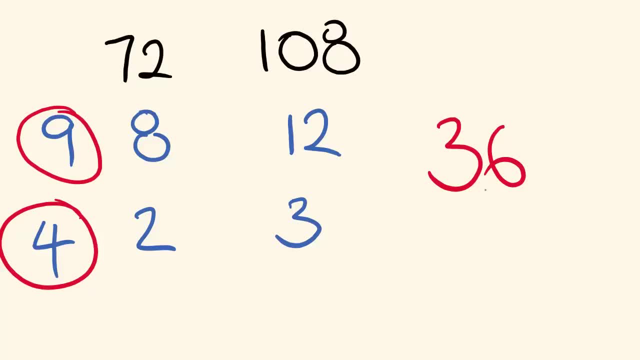 So I find this a lot neater, easier method of doing this. Anyway, thank you for watching. We'll see you next time. Bye Captions by GetTranscribedcom.